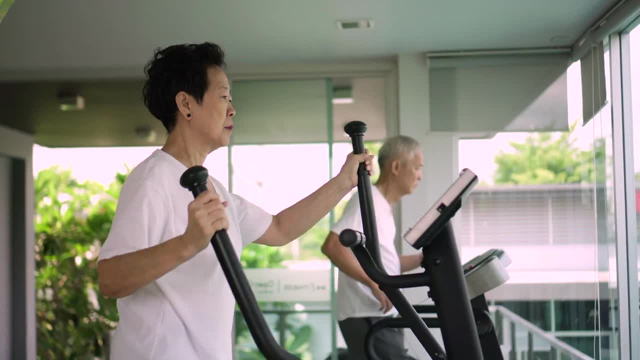 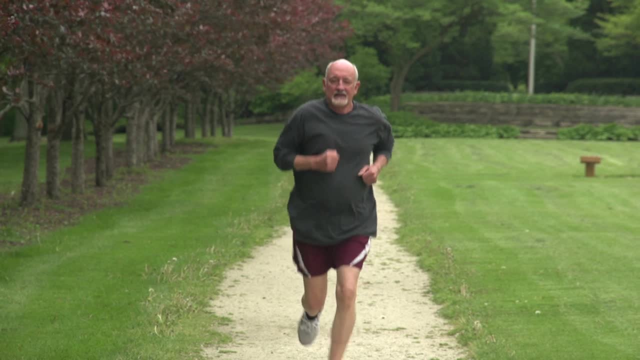 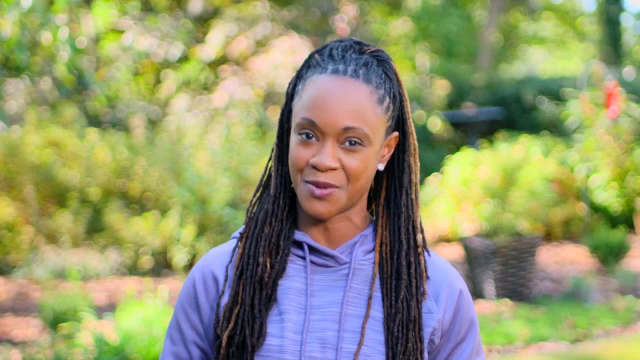 In this video, we're going to talk about how being physically active can play a vital role in helping you stay well, so that you can best support your loved one with cancer. You know better than anyone how hard it is to find time to get things done in addition to your caregiving responsibilities. 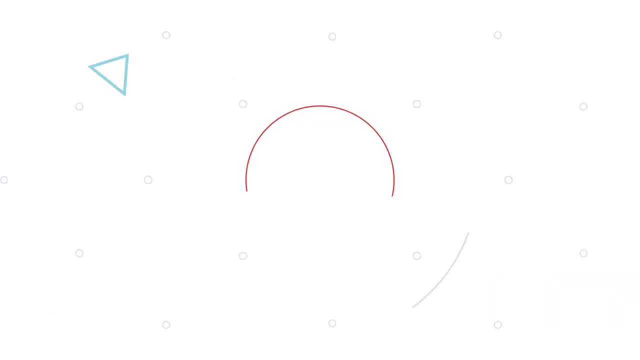 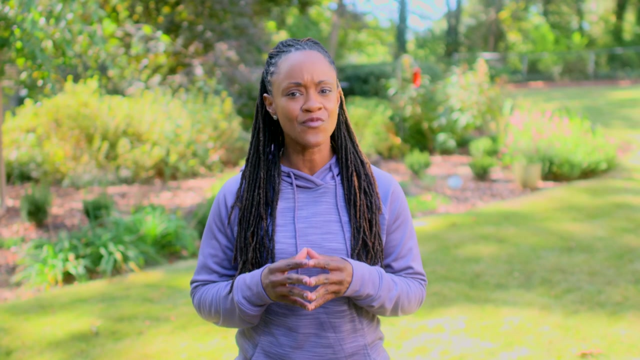 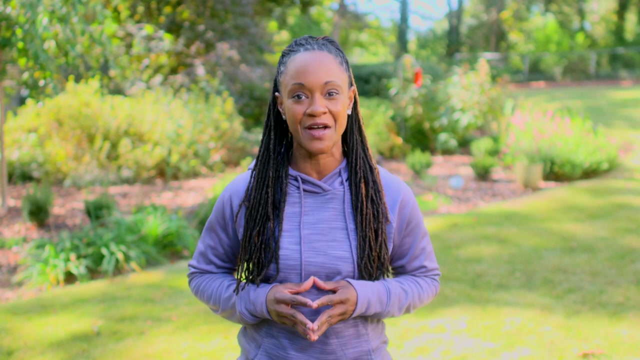 Taking time each day to commit to activity will help protect your immune system, give you energy and help you rest better at night. Research shows that regular activities can help you stay healthy. Regular exercise also helps lower anxiety and depression, which are feelings you may have experienced while providing care. 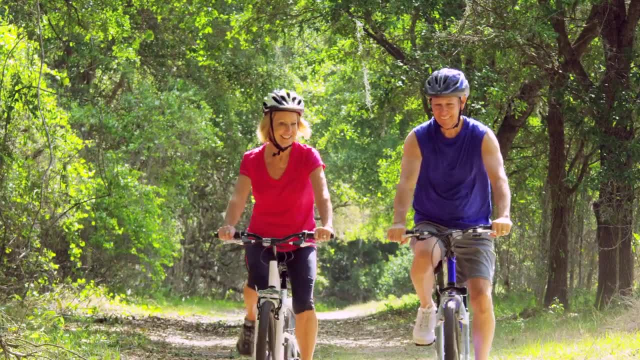 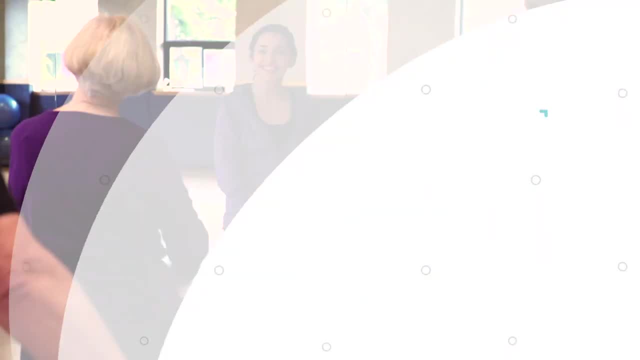 Whether you have been active prior to becoming a caregiver or whether you are just getting started, here are a few things to keep in mind to make it easier to meet your active living goals. First, start by committing to at least 30 minutes a day to get moving. 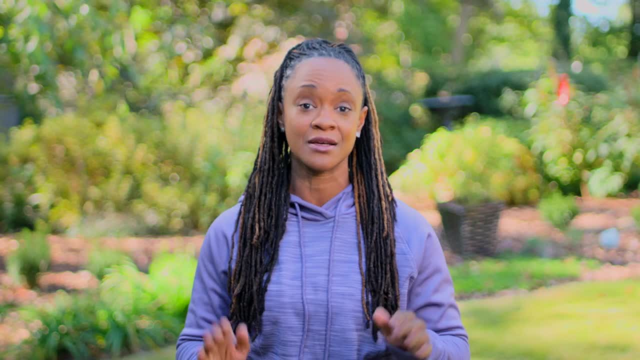 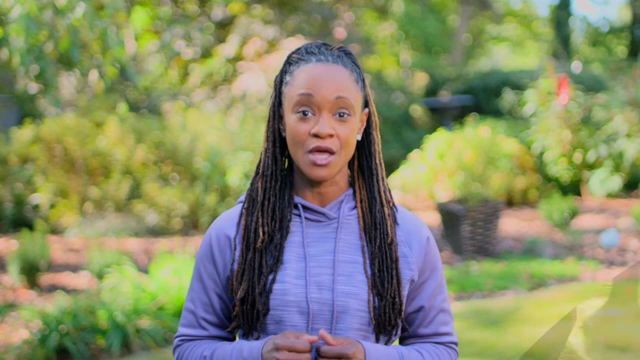 If you can do 30 minutes or more at a time, that's great. If not, even a small amount of activity during the day will help. If you can do 30 minutes or more at a time, that's great. This longer term commitment to stay working for a long term basis helps reduce stress and causedслittiness and makes you feel good and better. 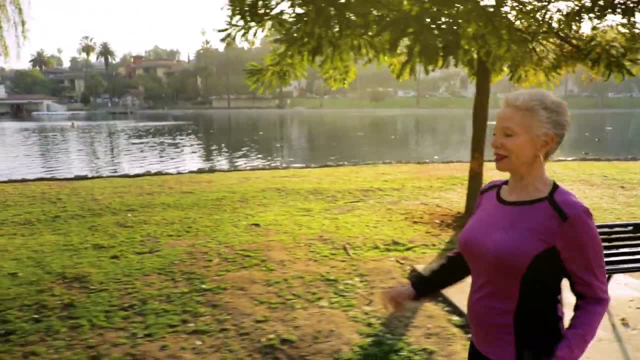 If you sand to this extent, that's not the best decision. Nice, talk is all there and take your time, rub this down and make sure you are burn sort of может make your body, diyor, Whether it's a brisk walk around the block or an air condition mall or doing a workout DVD or a video on Youtube. 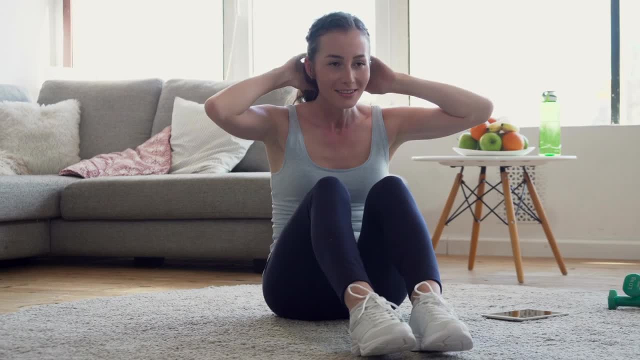 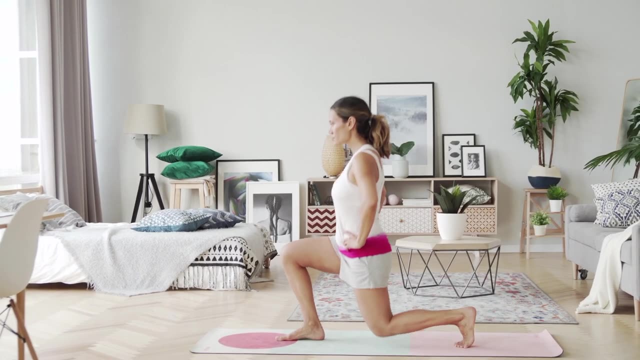 There are plenty of ways to be active even if you don't have a gym membership. There are many helpful and easy at-home workouts as well, where no weights are required. Staying together is an awesome way to stay in shape for such long an you. 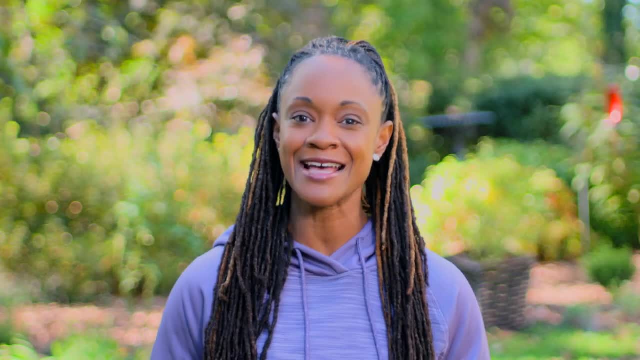 Just keep your balance. You know the muscle you take as you go out & on need more time to victimize physical activity. Staying focused REALLY Вс benefit of providing some additional emotional support Also, if it's possible. 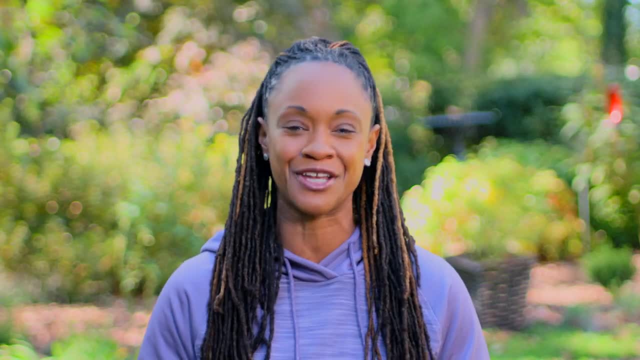 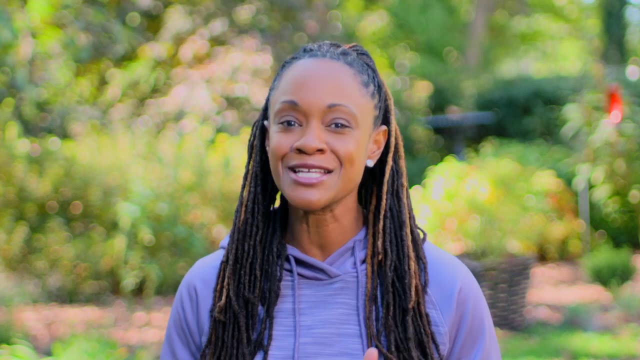 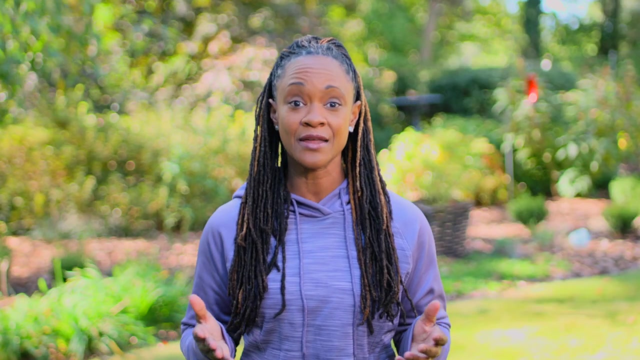 try to carve out some time to be active with the person you're caring for. It's important for individuals undergoing treatment to be active as best they can. We tend to be more motivated and are more likely to reach our goals when we take the team effort approach. You may find that you have so much going on at. 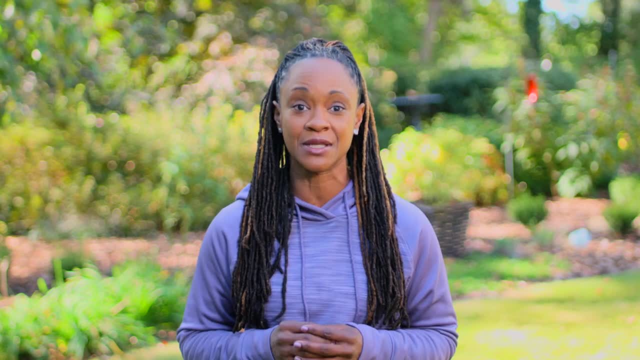 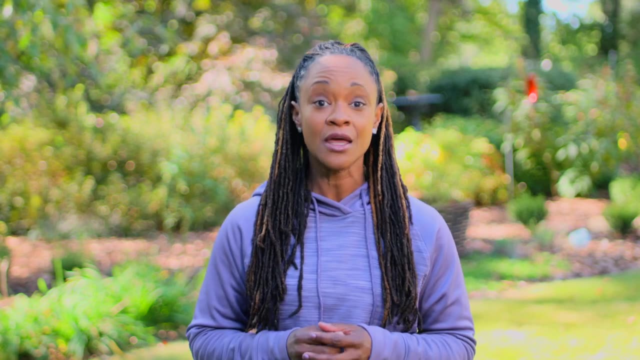 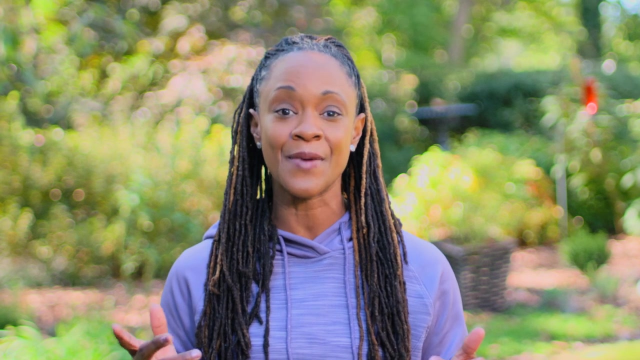 home and work in addition to your caregiving responsibilities, that it's difficult to take time out for a walk, a bike ride or whatever your favorite ways are to be active. If there are others who live in your home with you, don't hesitate to ask them for help Cooking and cleaning up after a meal. 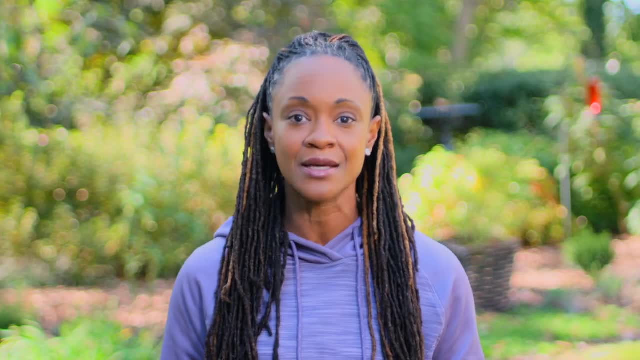 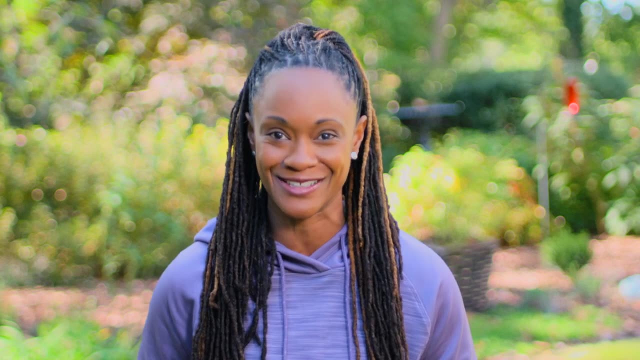 doing a load of laundry or doing the grocery shopping. Simply having someone help with these responsibilities can free up some much-needed time for you to be active On days when your loved one must spend an hour or more in the chemo infusion room. 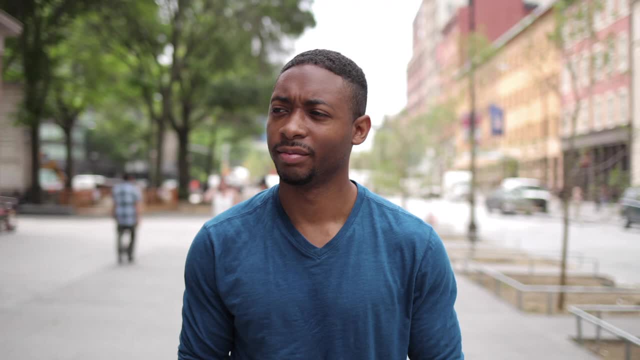 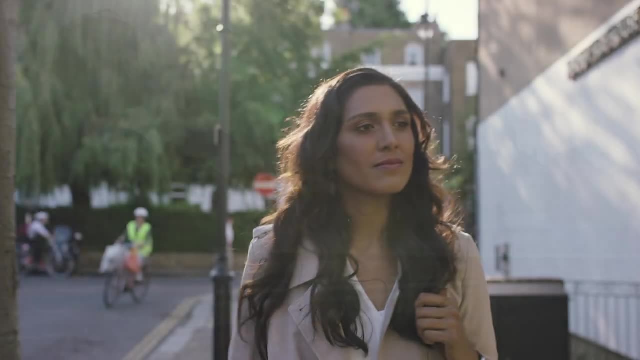 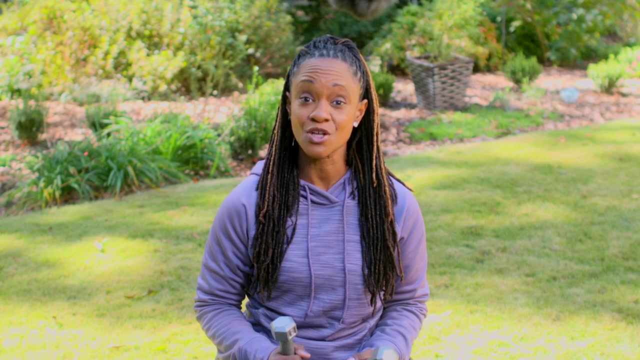 take that chance to walk around the hospital or outside, around the property. This break will help boost your energy level and will certainly make you feel good. And remember, getting a breath of fresh air outdoors is always good for the soul. Strength training is also something to think about as you may have to lift. 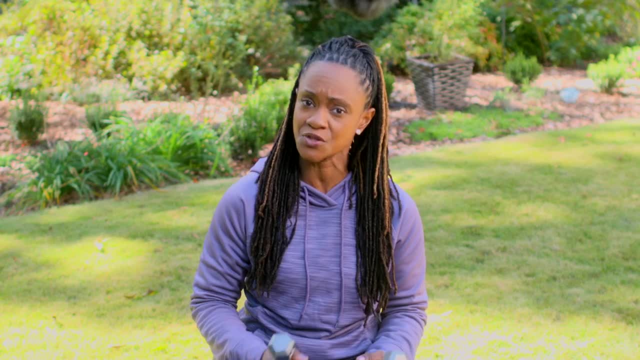 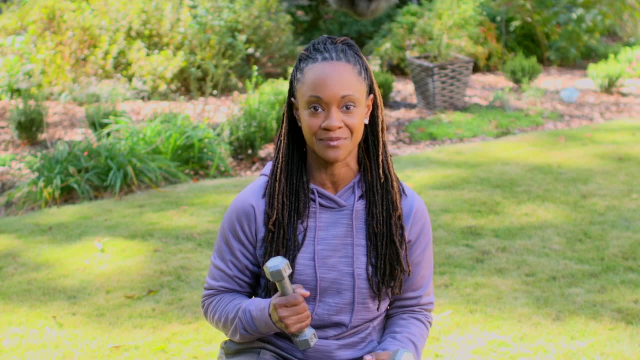 your loved one to help them move from the toilet to the bed or elsewhere. Increasing your strength will help make you more capable of assisting in the physical demands of your loved one. If you have any questions, feel free to contact us at healthcaregivingcom. Strength training can also help with balance support Think. 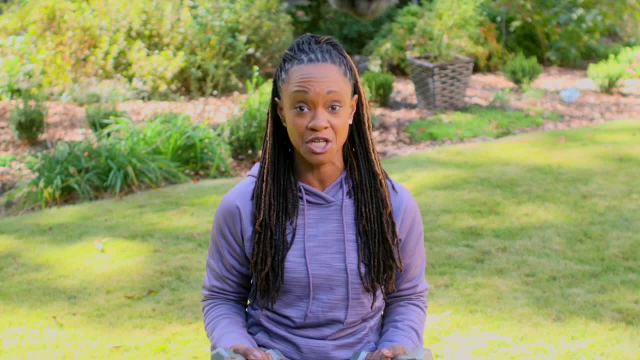 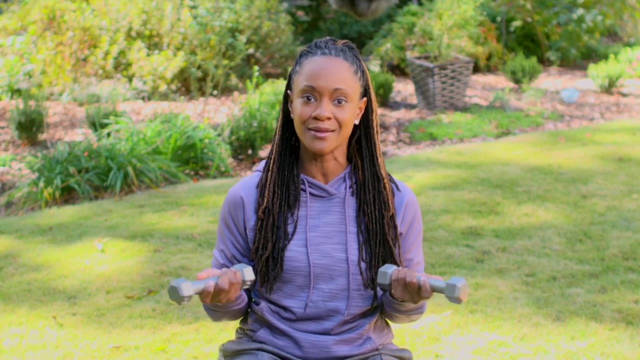 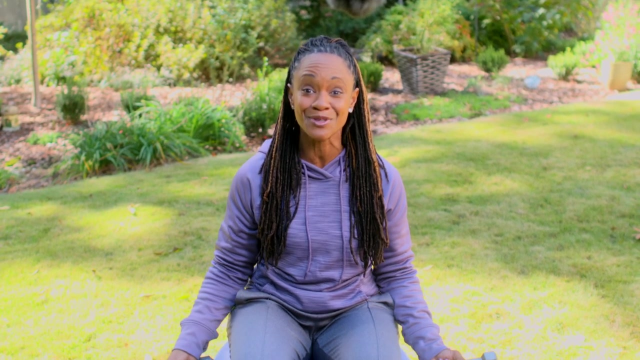 about adding weights to your routine. Doing squats, push-ups or even wall push-ups and stomach crunches can also help. Simple, affordable home equipment can be helpful as well. For instance, these small hand weights give you a little extra resistance and something to grasp. Or this stability ball makes a great aid. 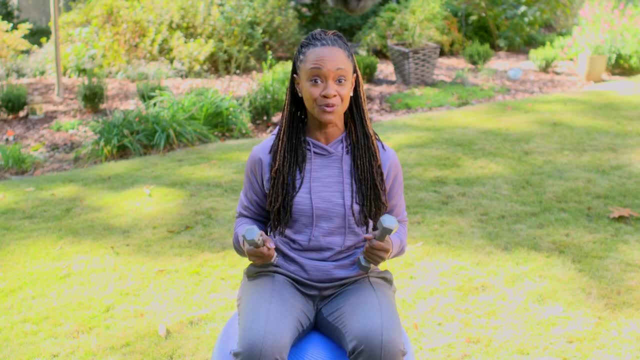 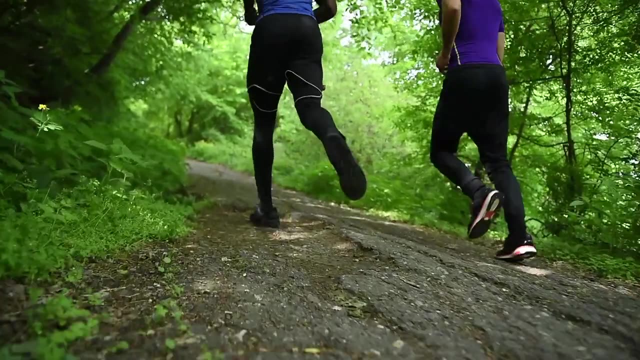 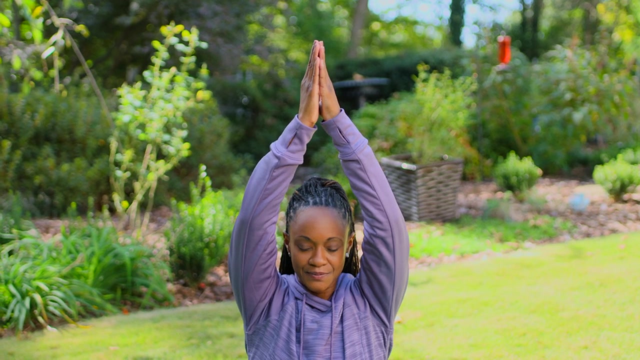 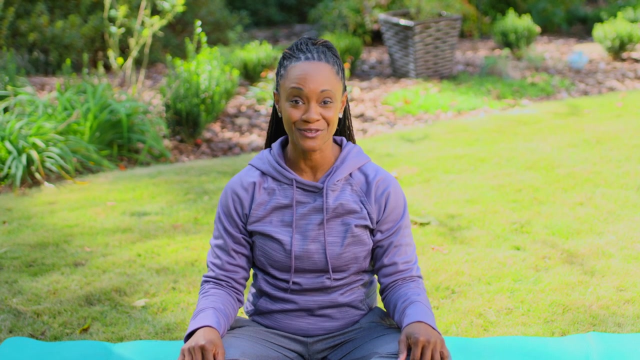 and allows for some versatility in your routine while building your body. It's a great way to build your body and your mind. Remember, always consult your physician if you have a medical problem or concerns prior to starting any workout regimen. That felt wonderful. Stretching and deep breathing throughout the day will slow. 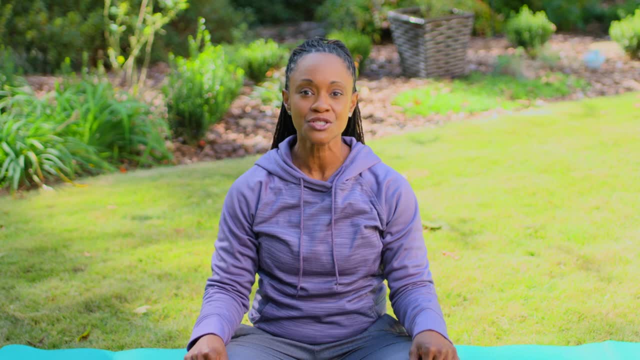 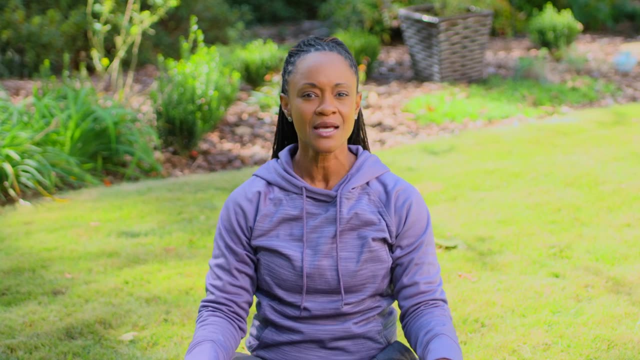 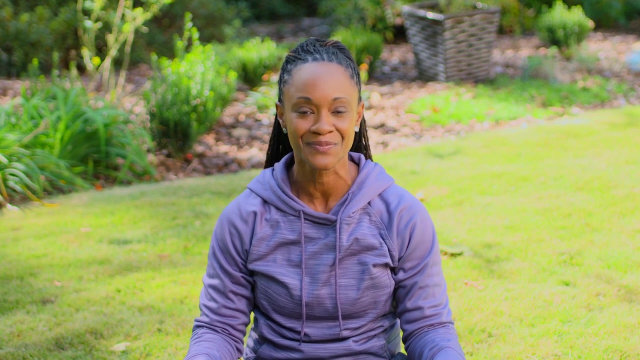 your stress response and help center you. Stretching will also help with your improve your flexibility, which again can be a big help if you need to lift your loved one. Taking small spurts of time to stretch and deep breathe can make a world of difference in your movements throughout the day. End each day by 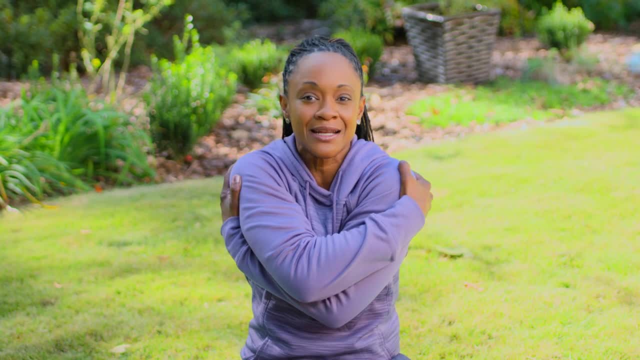 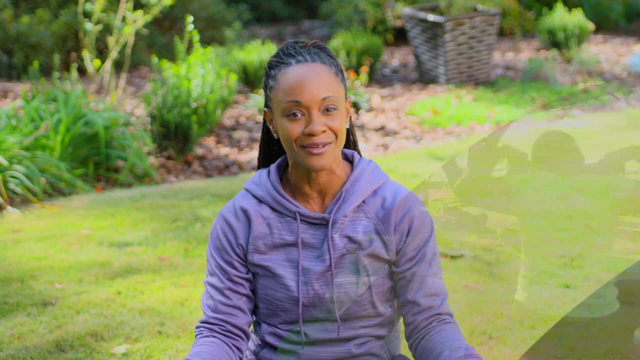 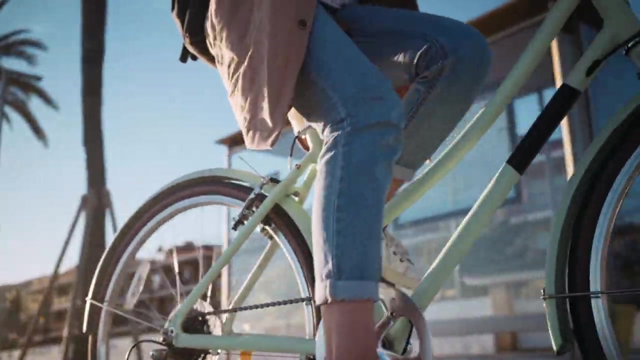 giving yourself a big hug, Take any moment to get a last little stretch in, as well as embrace yourself, acknowledging your need for support and love. So, as you can see, it's okay to be creative and have fun with it. There are a variety of options to get you moving and provide some change from the